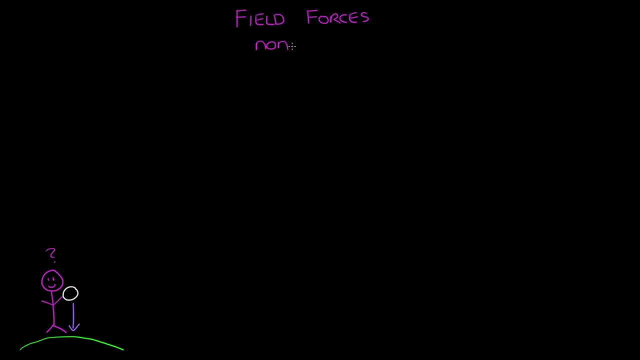 gravitational force is pulling the ball and gravity is a non-contact force. Non-contact forces don't have to touch an object to exert a force on it. Instead, these forces act over a region, So if an object is in that region, it will be affected by the force. In this case, the ball is. 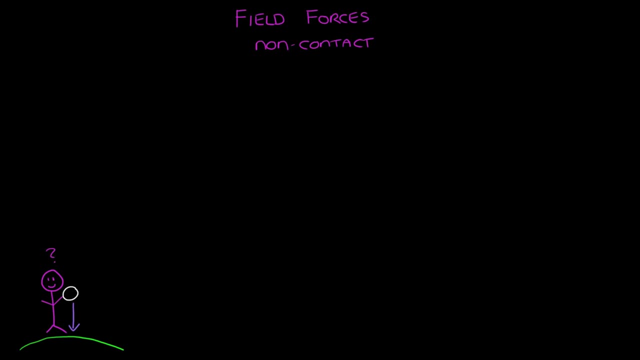 in Earth's gravitational field, and so it feels an attractive force towards the Earth and the ball falls to the ground. Field forces include non-contact forces such as electric, magnetic and, of course, gravitational forces. So since these forces are non-contact, they can exert a force on. 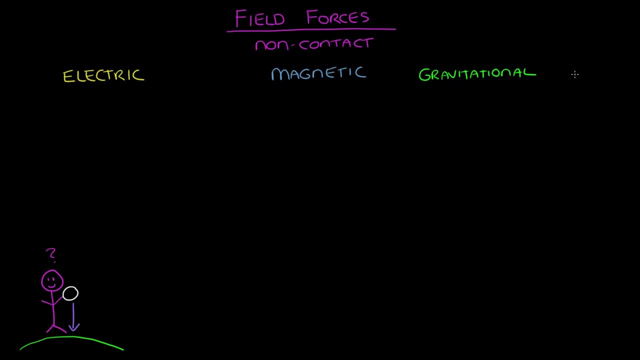 objects they aren't touching. But how do these objects know if there's a force between them? To explain these non-contact forces, scientists eventually developed the idea that these objects were surrounded by something called a field. So what is a field? A field extends through space from an object with certain 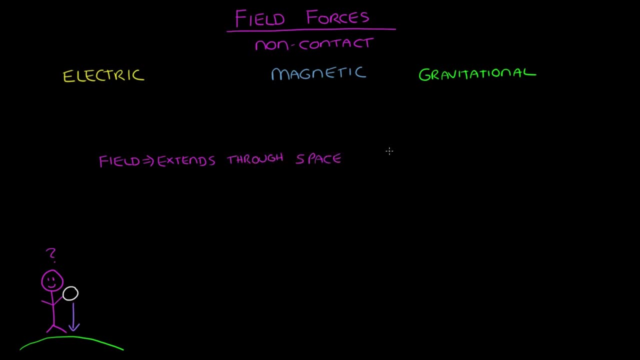 physical properties. What are those? Well, for gravitational forces. these affect objects with mass. So any object with mass has a gravitational field surrounding it. If it's in a non-contact force, it can exert a force on it. So if an object is in 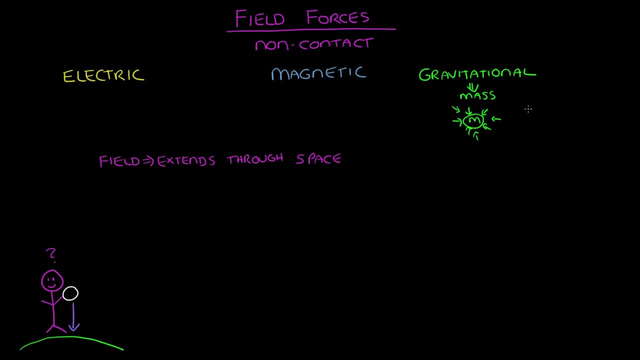 it that points towards the object center. The further you move away from the object, the less dense the field and weaker the field becomes. Electric forces affect charged objects, so an electric field surrounds any object with a net charge, and the direction of this field will. 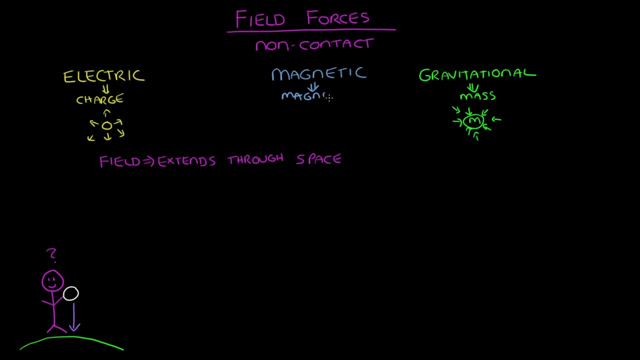 depend on the charge. Magnetic fields will affect magnets and any other material with magnetic properties. Each spot on a field has two things associated with it: magnitude and direction, and these help us predict what forces objects will experience when they're in the field. So let's 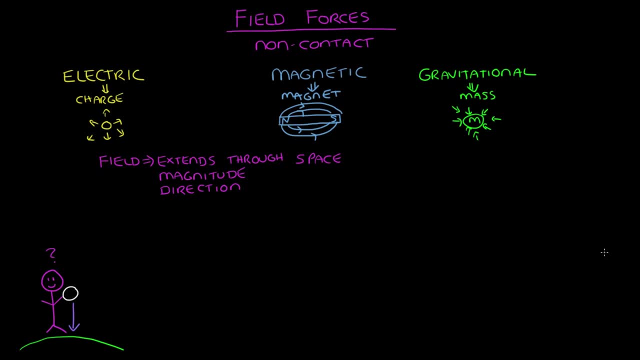 look at an example to help understand this. Say, we have a planet. Now the planet has a lot of mass, so we know it's going to be surrounded by a gravitational field that points towards the center of the planet. I can draw these little field lines that show the direction of the field.